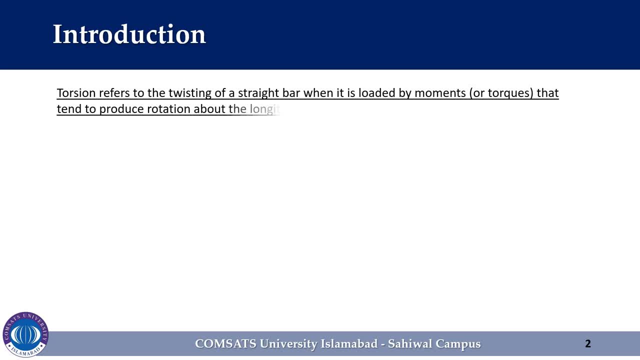 or torques that tends to produce rotation about the longitudinal axis of the bar. For instance, when you turn a screwdriver, your hand applies a torque T to the handle, as shown here in figure, and twists the shank of that screwdriver. Other examples of bar. 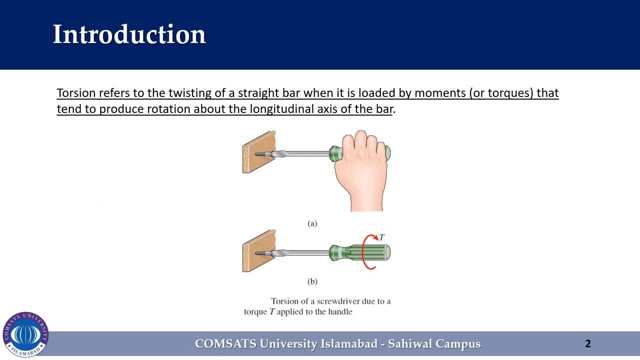 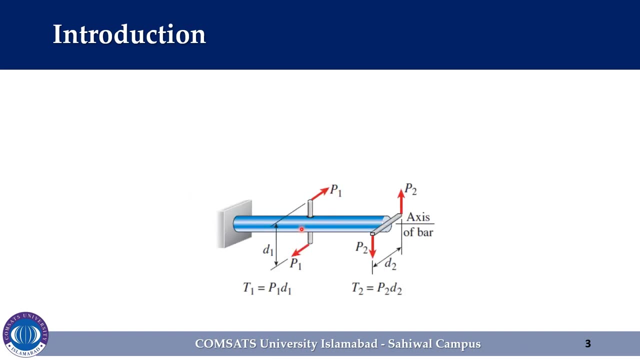 in torrion are drive shank In automobiles, axles, propeller shafts, steering rods and drill bits. However, for better understanding, an idealized case of torrional loading is pictured here, which shows a straight bar supported at one end and loaded by two pairs of equal and opposite. 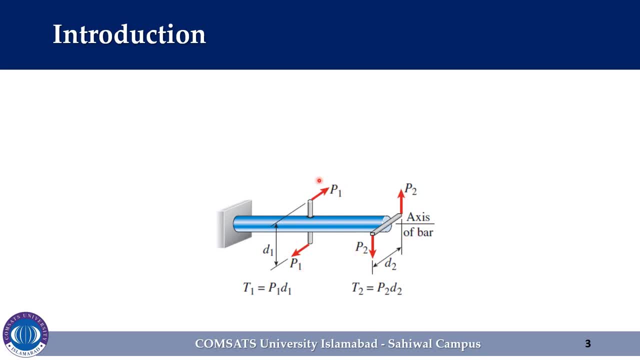 forces. The first pair consists of the forces P1 acting near the midpoint of the bar, and the second pair consists of the forces P2 acting at the end. This forms a couple that tends to twist the bar around its longitudinal axis. As we know from statics, a moment of a couple is equal to the product of one of the forces. 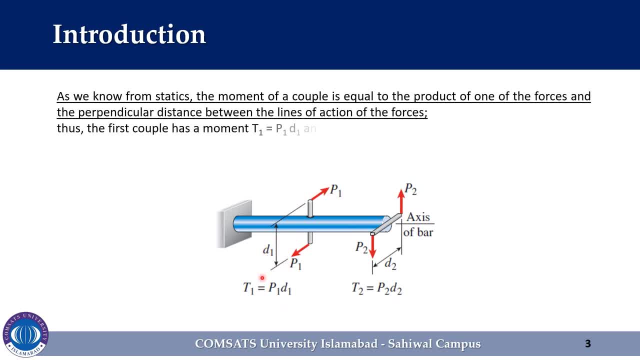 and the perpendicular distance between the lines of action of the forces. Thus, the first couple has a moment that is represented with: T1 is equal to force P1 and the distance D1, and in the same way, the second couple has the moment T2 is equal to T2- D2.. This equates to the Deadline distance of the force mil shaft and the distance of thealth versus the force D Due. so these numbers as shown here. The tutorials are less significant via video هنا, and the links to these are documented in disciple. This concludes our insight in SatyaStruxuralcom. 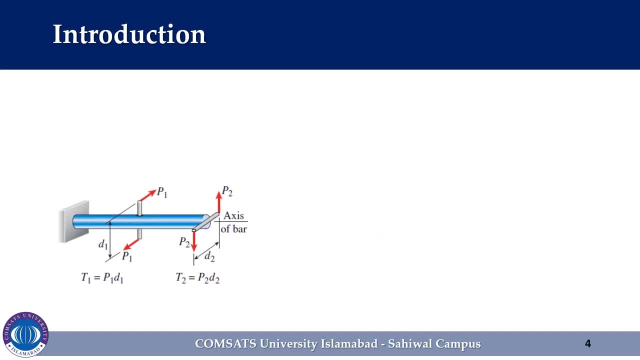 The SI unit for movement is the Newton meter. The movement of a couple may be represented by a vector in the form of a double-headed arrow. The arrow is perpendicular to the plane containing the couple And therefore, in this case, both arrows are perpendicular to the axis of the bar. 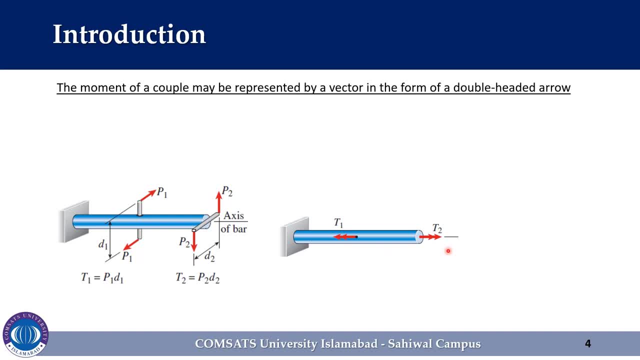 The direction or sense of the movement is indicated by the right-hand rule for movement vectors, Namely, using your right hand, let your fingers curve in the direction of the movement and then your thumb will point out the direction of the vector. However, an alternative representation of the movement is a curved arrow acting in the direction of rotation. 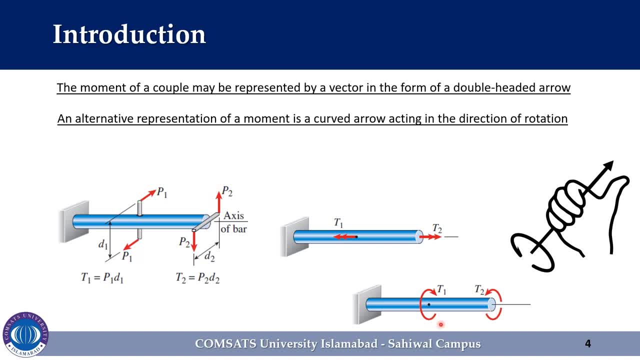 Both the curved arrow and vector representations are in common use. The choice depends upon convenience and personal preferences. So we can say that moments that produce twisting movement of a bar, such as the moments T1 and T2 here in figure, are called torques or twisting moments. 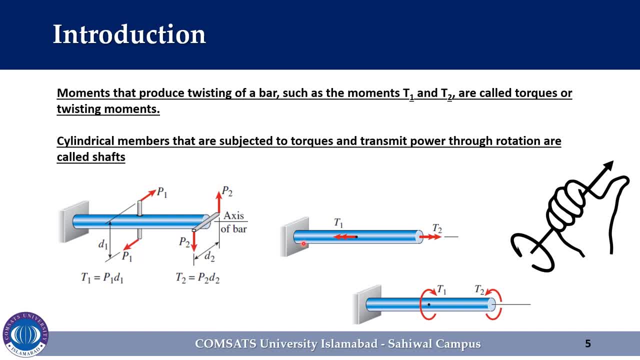 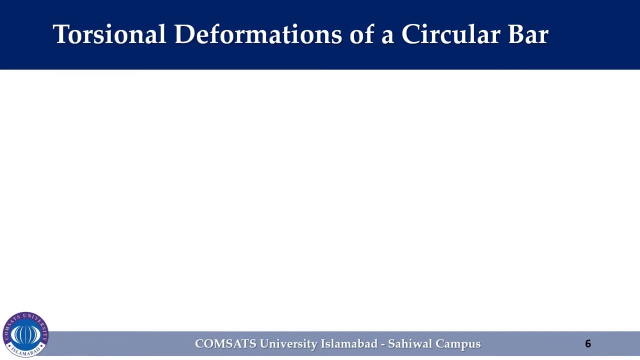 And cylindrical members that are subjected to torques and transmit power through rotation are called shafts, For instance the drive shaft of an automobile or the propeller shaft of a ship. After brief discussion on torrion, now we will discuss about torrional deformations of a circular bar. 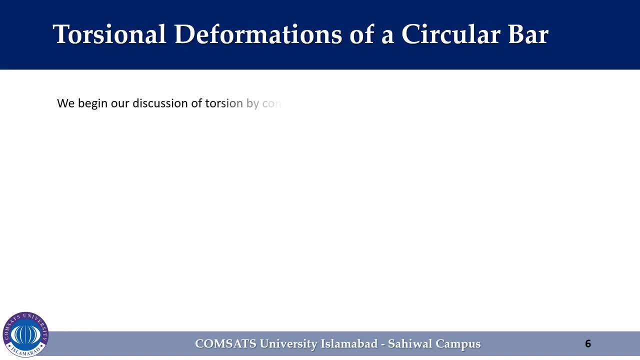 We begin our discussion of torrion by considering the arithmetic bar of circular cross-section twisted by torques T acting at the ends, as shown here in figure. Since every cross-section of the bar is identical and since every cross-section is subjected to the same internal torque T, 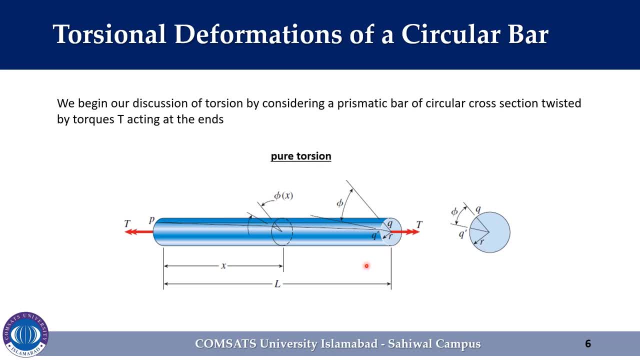 we say that the bar is in pure torrion From considerations of symmetry. it can be proved that cross-sections of the bar do not change in shape as they rotate about the longitudinal axis. In other words, all cross-sections remain plain and circular and are ready, remain straight. 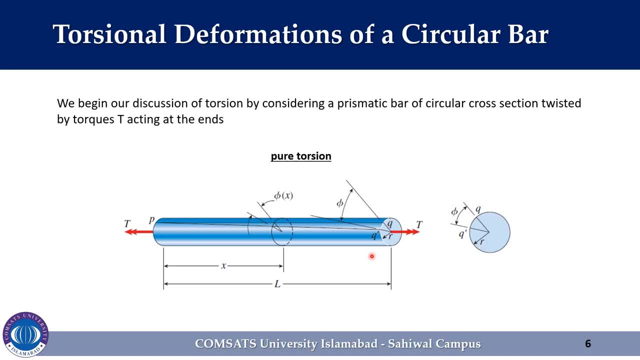 Furthermore, if the angle of rotation between one end of the bar and the other is small, neither the length of the bar nor its radius will change. However, to add, in visualizing the deformations of the bar, imagine that the left-hand end of the bar is fixed in position. 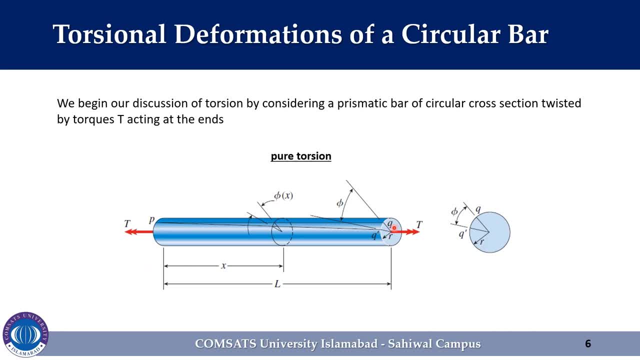 Then, under the action of the torque, the right-hand end will rotate with respect to the left-hand end Through a small angle, phi, known as the angle of twist or angle of rotation. Because of this rotation, a straight longitudinal line- PQ- on the surface of the bar will become a helical curve- PQ'. 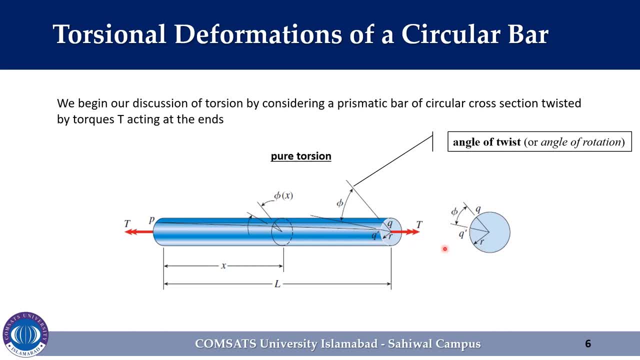 where Q' is the position of the point Q after the end cross-section has rotated through the angle phi. The angle of twist changes along the axis of the bar and at intermediate cross-sections it will have a value of phi that is in between 0 at the left-hand end and phi at the right-hand end. 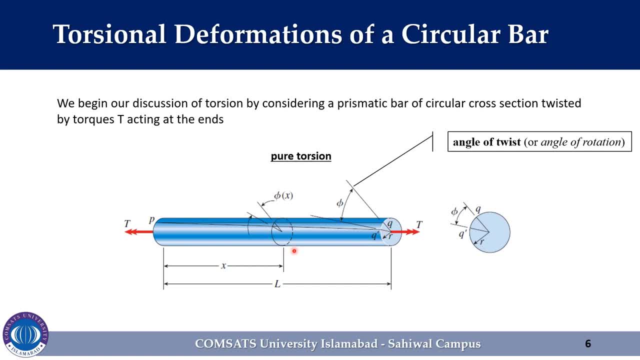 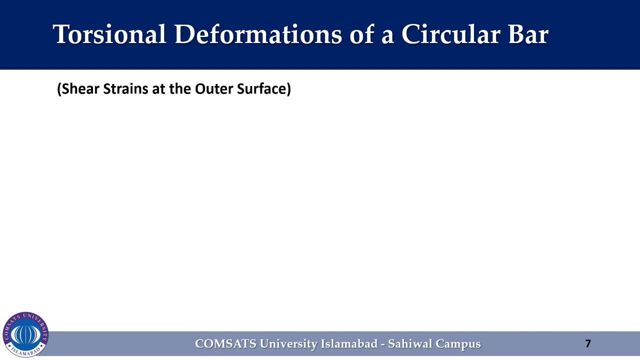 If every cross-section of the bar has the same radius and is subjected to the same torque or peartorian, the angle phi will vary linearly between the ends. Now we will discuss about shear stains at the outer surface. Now consider an element of the bar between two cross-sections, distance dx apart. 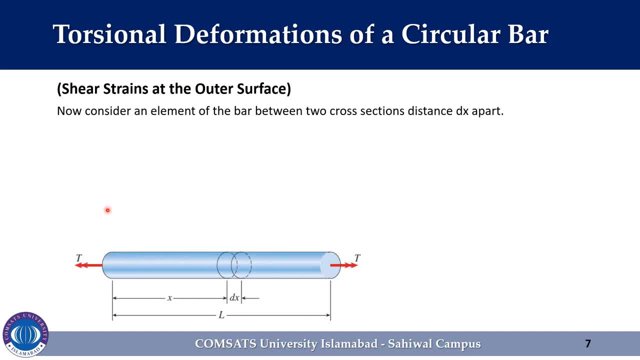 This element is shown in large in figure here. On outer surface we identify a small element represented with ABCD, which sides AB and CD that initially are parallel to the longitudinal axis. During twisting of the bar, the right-hand cross-section rotates with respect to the left-hand cross-section. 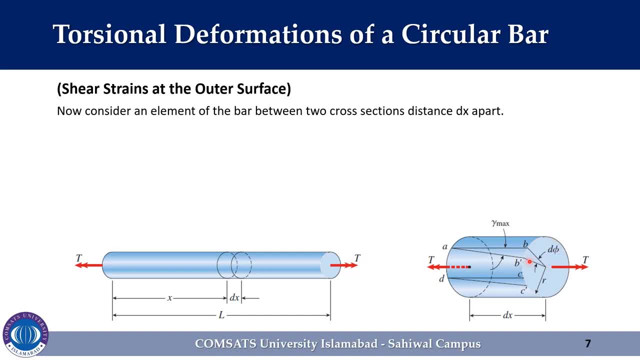 Through a small angle of twist d phi, The points B and C moves to B' and C' respectively. The lengths of the sides of the element which is now element A, B', C' and D do not change during this small rotation. 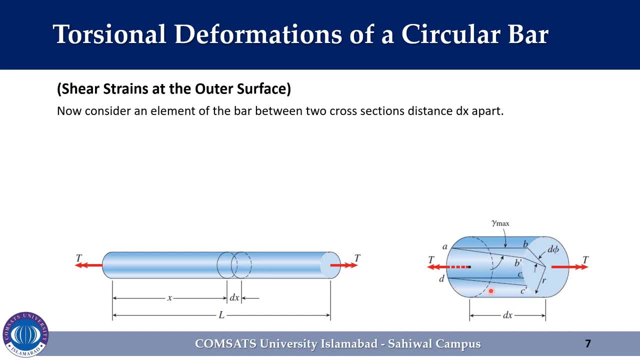 However, the angles at the corners of the element are no longer equal to 90°. now The element is therefore is in a state of pure shear, which actually means that the element is subjected to shear stains but no normal strain. The magnitude of shear stain at the outer surface of the bar denoted gamma max. 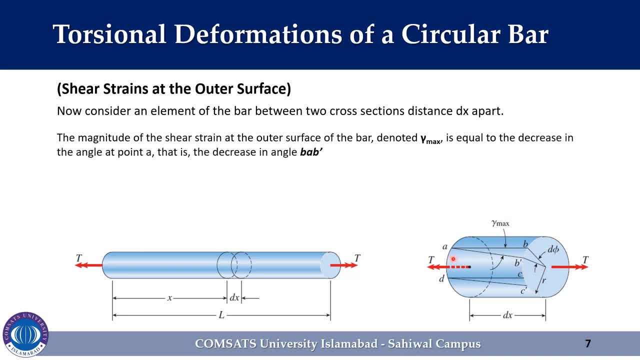 and is equal to the decrease in the angle at point A, that is, a decrease in angle BA and B' So we can express this equation as gamma max is equal to BB' over AB, Where gamma max is measured in radians and BB' is the distance through which point B moves. 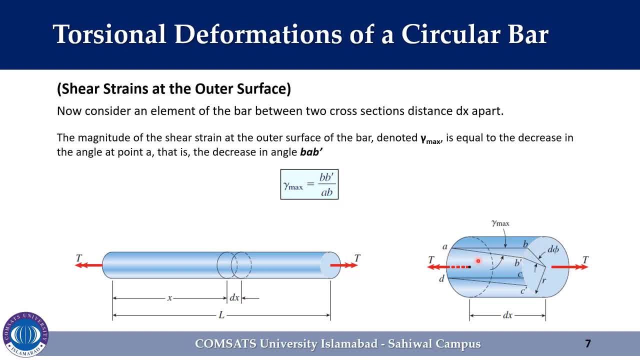 In the same way, AB is the length of the element equal to dx, With R denoting the radius of the bar. we can express the distance BB' as R d phi, Where d phi also measured in radius. Thus the preceding equation becomes: gamma max is equal to R d phi over dx. 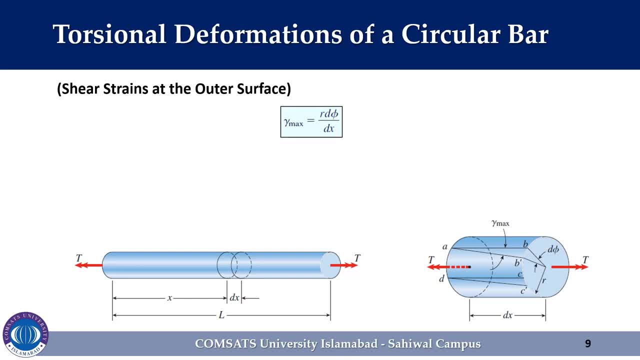 So this equation relates the shear strain at the outer surface of the bar. We can express the shear strain at the outer surface of the bar to the angle of twist. However, the quantity d phi over dx is the rate of change of the angle of twist. phi. 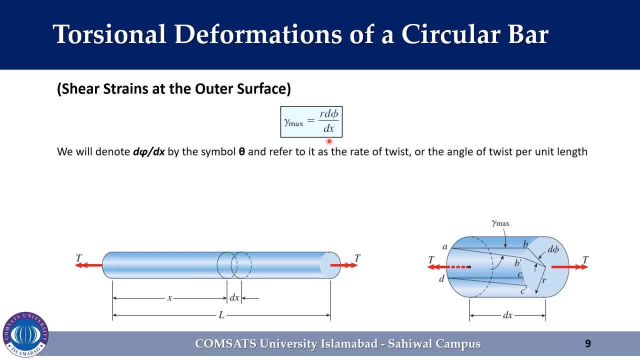 with respect to the distance x measured along the axis of the bar, We can express d phi over dx by the symbol theta and refer to it as the rate of twist or the angle of twist per unit length. With this notation, we can now write the equation. 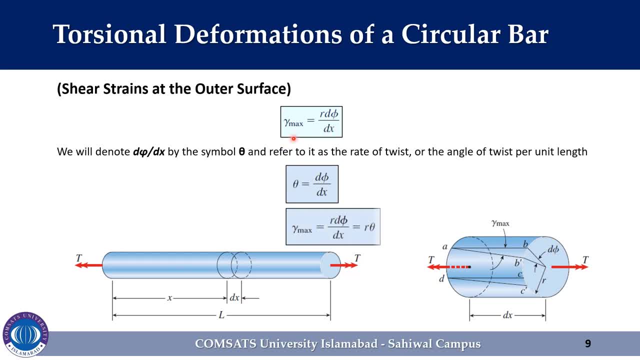 for the shear strain at the outer surface of the bar as follows: The maximum is equal to R d phi over dx. and now we can express it as: by replacing the d phi over dx with angle theta, The equation becomes R theta. In our previous discussion, 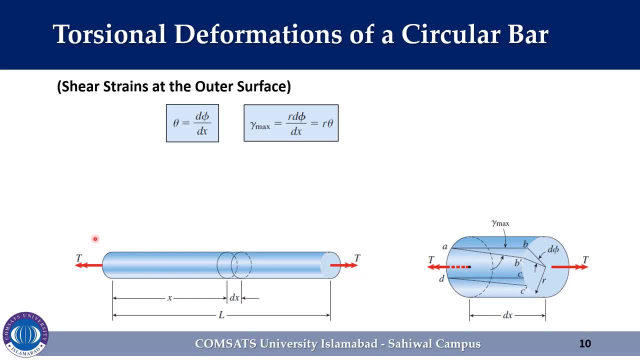 for convenience. we discussed a bar in paired torrion. However, both equations are valid in more general cases of torrion, Such as when the rate of twist theta is not constant but varies with the distance x along the axis of the bar. In the special case of paired torrion, 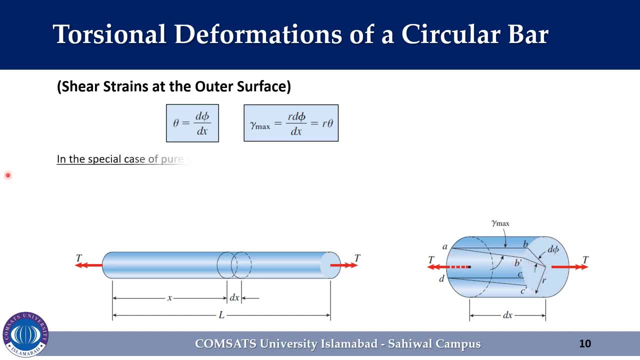 the rate of twist is equal to the total angle of twist, phi, divided by the length, L. Now we can express theta as phi over L. Therefore, for paired torrion only we obtain the expression as mega maximum is equal to R theta, and now, in this case, theta replaced with phi over L. 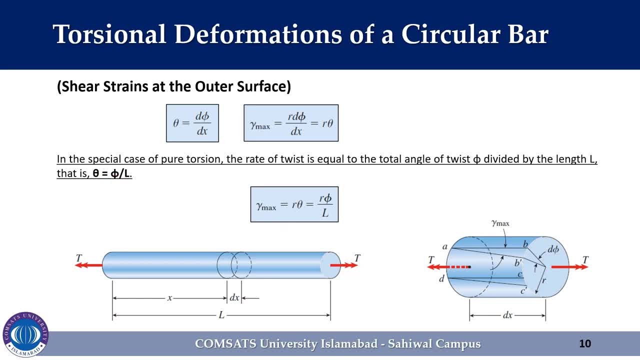 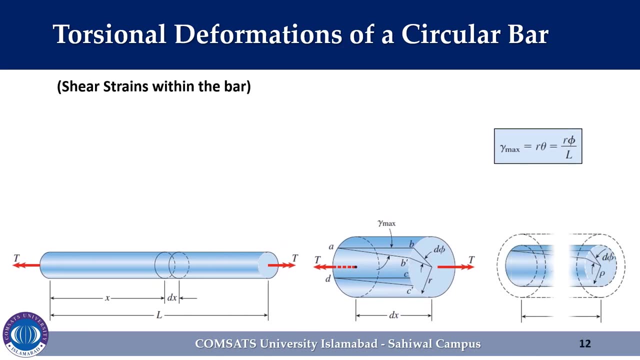 And this equation becomes R phi over L. So after discussing about shear strain at the outer surface, now we will study about shear strain within the bar. The shear strain within the interior of the bar can be found by the same method used to find the shear strain. 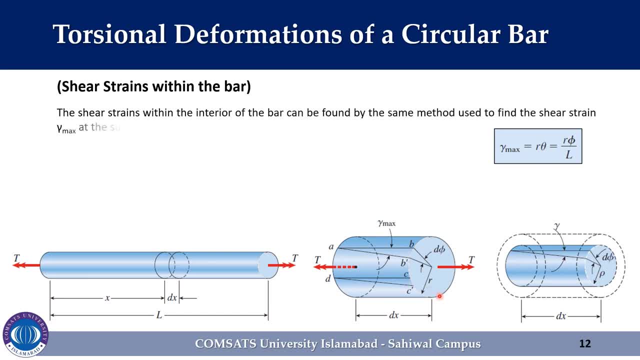 gamma maximum at the outer surface, Because ready in the cross sections of a bar, remains straight and undistorted during twisting. We see that the preceding discussion for an element ABCD at the outer surface will also hold for a similar element situated on the surface of an interior cylinder of radius rho. 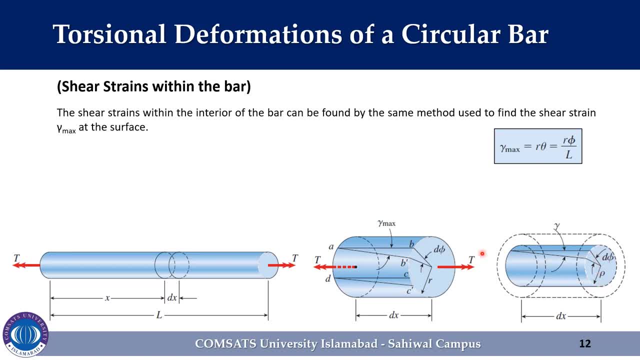 This interior element, also in pair shear, with the corresponding shear strain given by the equation gamma is equal to rho theta, And this equation can now be represented as rho over R gamma maximum, The radius R replaced with radius of interior cylinder rho and the length L replaced with